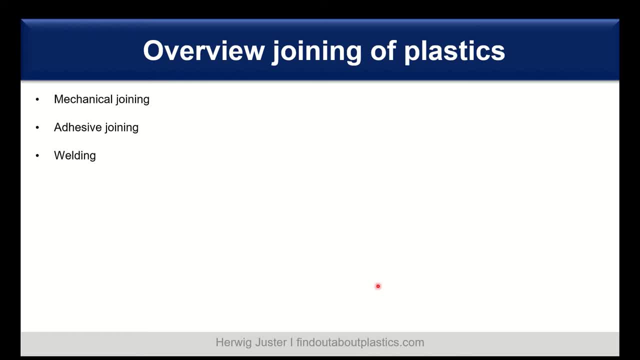 Ok, let us start with the overview of joining of plastics. There are three main methods how to join plastics. You can have a mechanical joining using a plier, Screws and bosses, either directly or in molded into your part. You can use adhesive joining using glues. 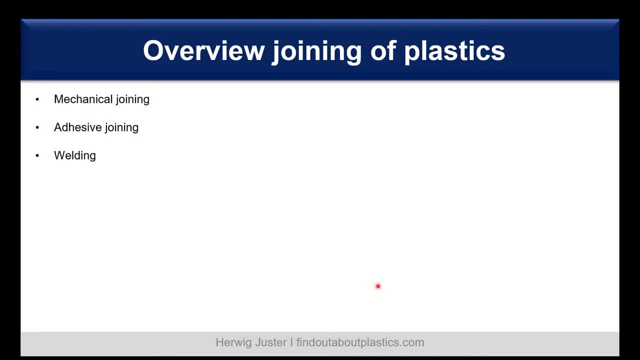 And you can use welding techniques, And among the welding we can distinguish several different techniques So we can have vibration welding, ultrasonic welding, high frequency welding, extrusion, hot air welding, hot plate And laser welding using near infrared, And this is where we put the focus of today. 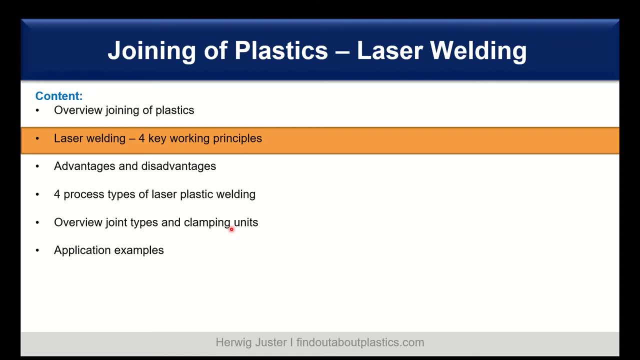 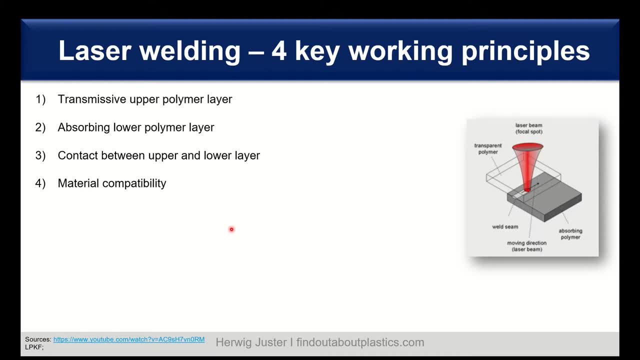 Let us continue with laser welding. the four key working principles. So what are the four key working principles? So first we need to have a transmissive upper layer. We need an absorbing lower layer. Then we need a good contact between the upper and the lower layer. 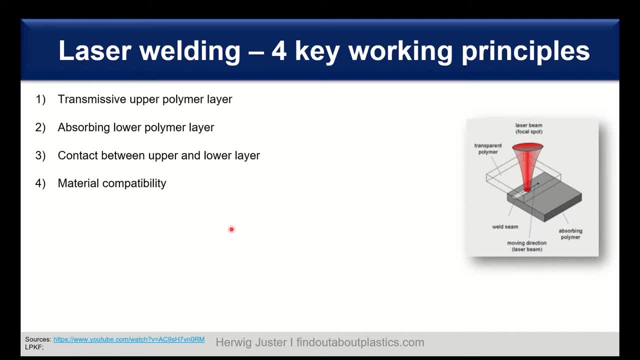 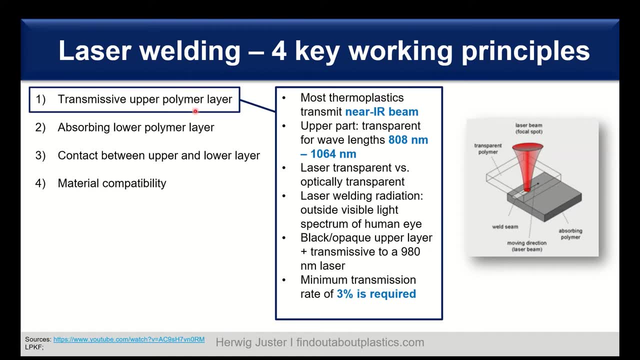 And we need to have the right material compatibility. So when we have a closer look at the transmissive upper polymer layer, So most thermoplastics transmit near infrared beam And the upper layer needs to be transparent in a wavelength around 800 nanometer to 1064. 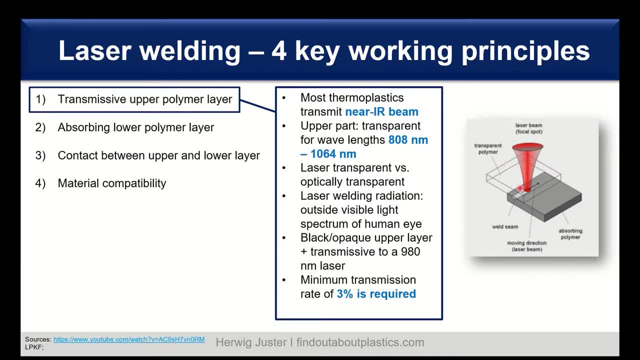 And this is also shown here. So we have here our transparent polymer upper layer and absorbing polymer layer, And here it is important to notice laser transparent versus optically transparent. So although this part can be black or opaque, it is still transmissive to infrared. 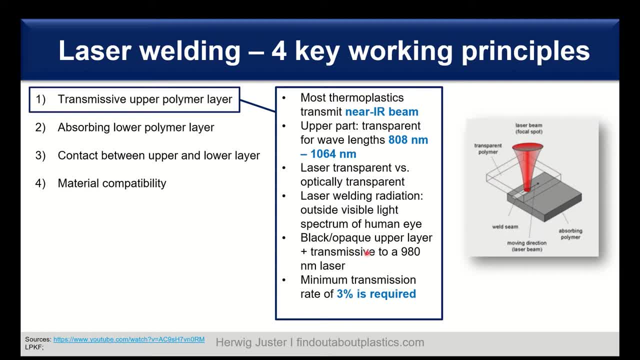 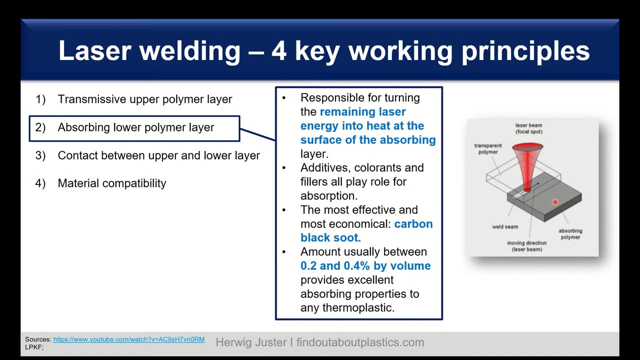 So, for example, what I have shown here, So we can have a black opaque layer and still transmissive to a 980 nanometer laser. However, we need a minimum transmission of 3%. Then the absorbing lower layer. So the main job of the absorbing layer is to turn the remaining laser energy into heat. 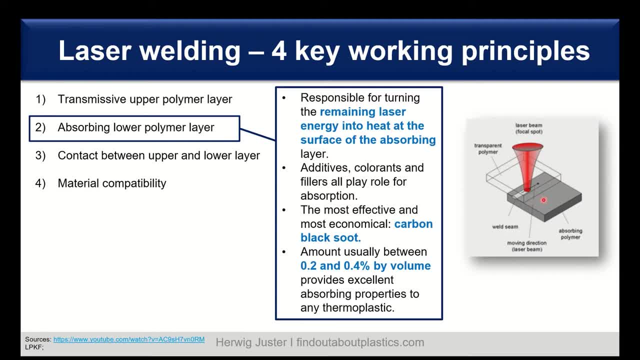 And this heat will melt then the absorbing layer And also transfer this heat to the transparent layer And can so enable the joining. And here, in the absorbing layer, additives, colorants and fillers play a key role for the absorption, And the most effective and most economical filler is carbon black soot. 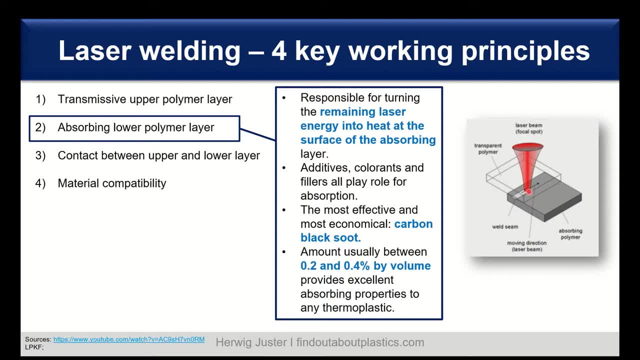 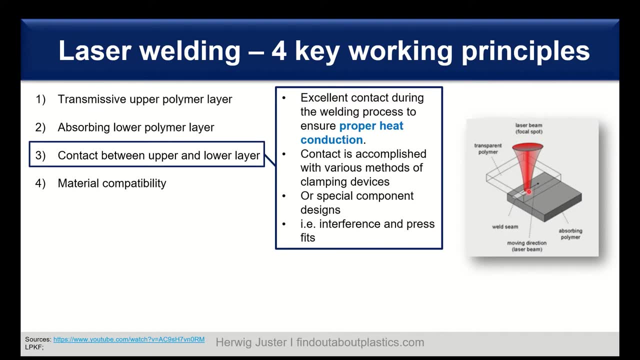 And you use around 0.2 to 0.5 for bi-volume And you can have already excellent absorbing properties. Then the contact between the upper and the lower layer. So we need to ensure the proper contact to have a good conduction of the heat. 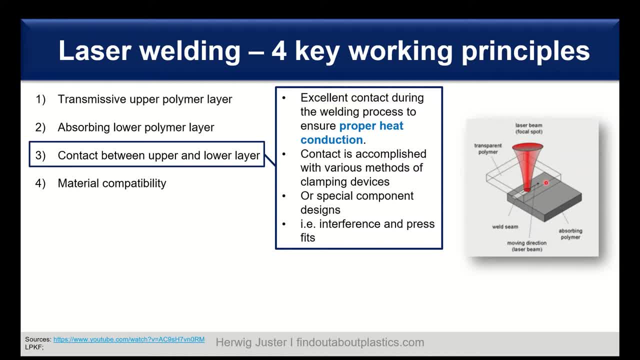 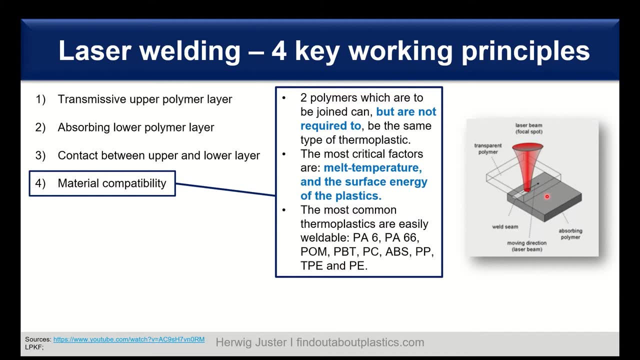 And the contact between those two layers is achieved by using different clamping methods And there are also special component designs. And then also the material compatibility. So you can have the case that you have two polymers which you want to join And they can but are not required to be the same type of thermoplastic. 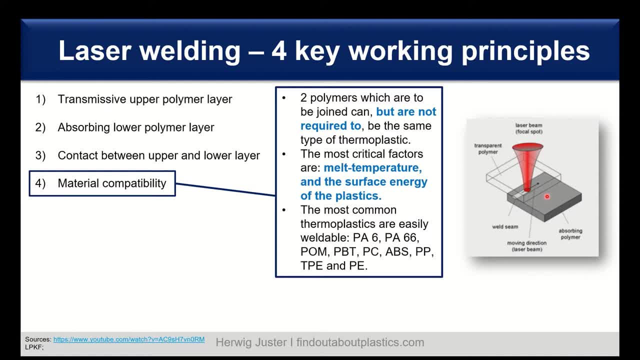 So the most critical factors here are, as already previously mentioned, melt temperature, So the transparent polymer and absorbing polymer need to have the same temperature. And also the surface energy of the plastics play a role. When we look, most common thermoplastics are easily weldable. 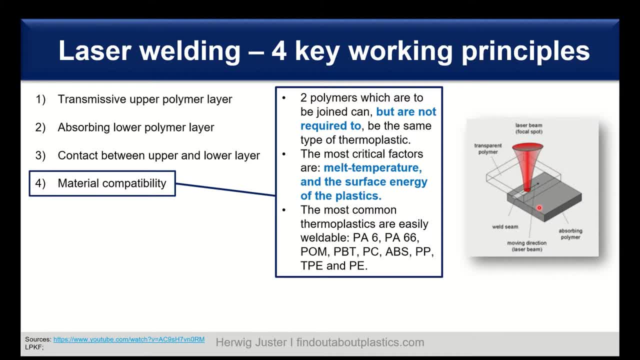 So the nylons, like polyamide 6,, polyamide 66,, POMs, PPT, polycarbonates, ABS, polypropylene, And also elastomers such as thermoplastic elastomers and other polyolefins. 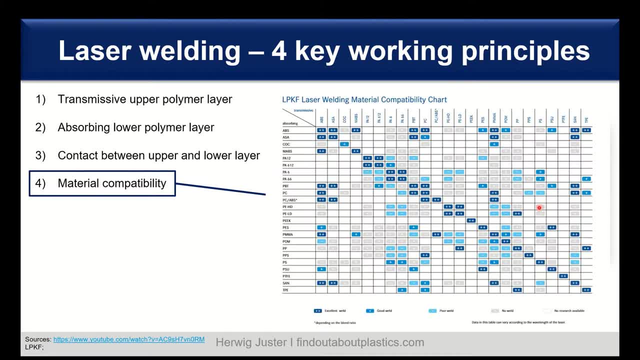 Here is useful to use so called material compatibility charts. Here is an example from a company, LPKF, And here you can have a look when you have now, the transmissive layer is a PA6. And the absorbing layer is also PA6. You can see this works pretty well. 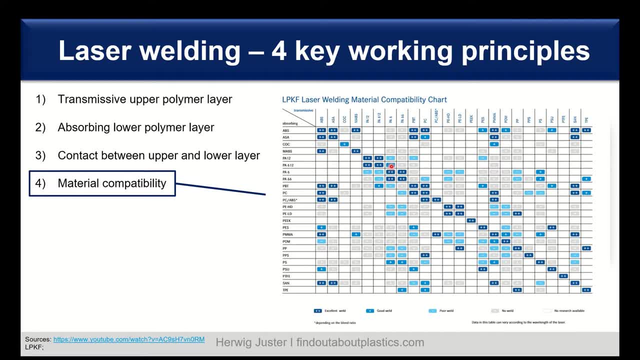 And when you go now to a PA6 transfer As absorbing layer, it also works. And when you go to a PA66 as absorbing layer, You have the same effect like a PA6.. And when you change now the transmissive layer to a PA66. 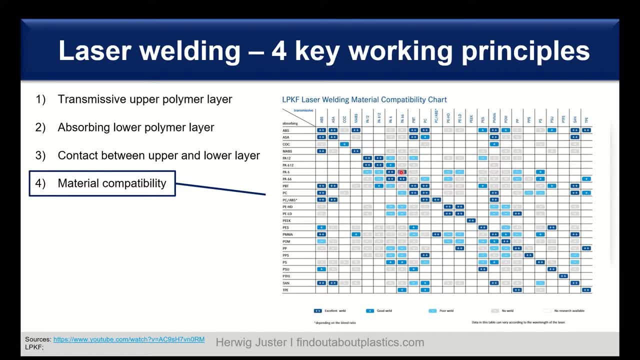 And use a PA6 as absorbing. this also works. So you see, it is really the polymer itself, And the melt temperatures of the polymer play here the key role, And such charts can help you to in material selection also to align the polymers. 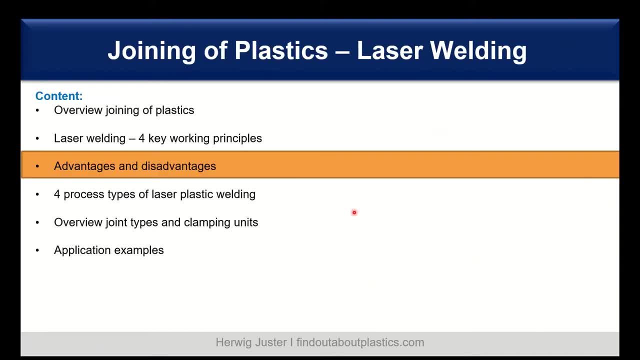 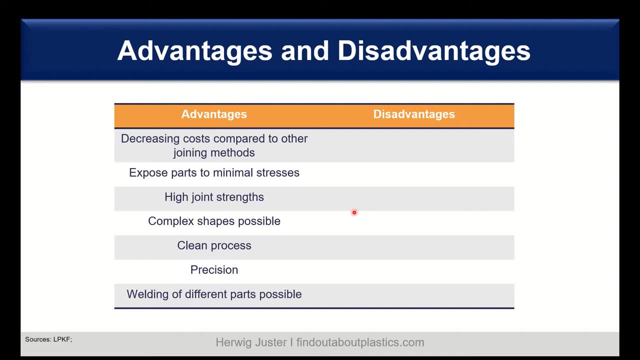 Ok, Let's discuss the advantages and disadvantages of laser welding. Let's start with the advantages first, And one of the biggest is the lower costs compared to other joining methods. So when you think you have no consumables, And also the maintenance is a minimum, 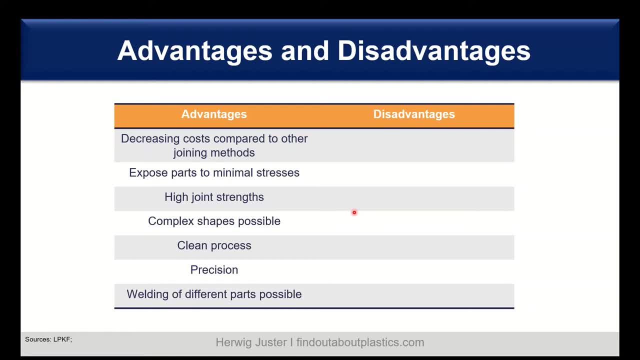 And you have also fewer failed parts. Then also the exposure of the parts to stress is minimum. So you have localized heat And this allows also to join and weld sensitive applications. Then we can achieve high joint strength. There are several tests like this pull test. 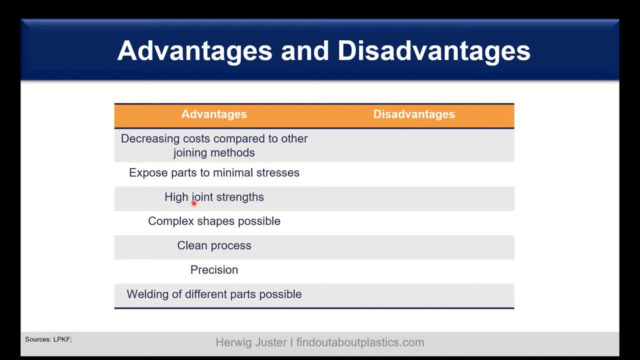 And there is the aim that the weld strength is bigger than the parent material. So when you pull them apart You should really have the parent material attached to the weld. Then complex shapes are possible Because the laser is always moving relative to the joint. 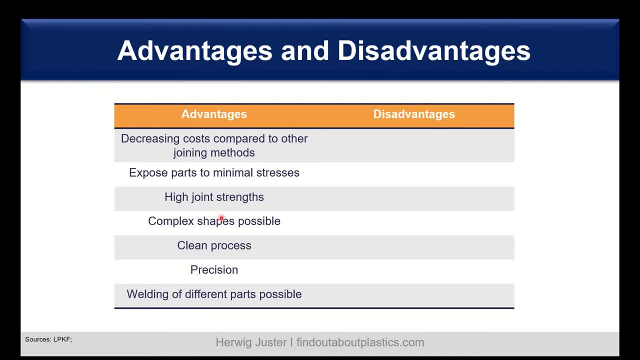 Then it's a very clean process, So you have no particles which can be removed, And also the high precision is an advantage, So you can have really thin welds, such as 2 microns, And welding of different parts and materials possible. 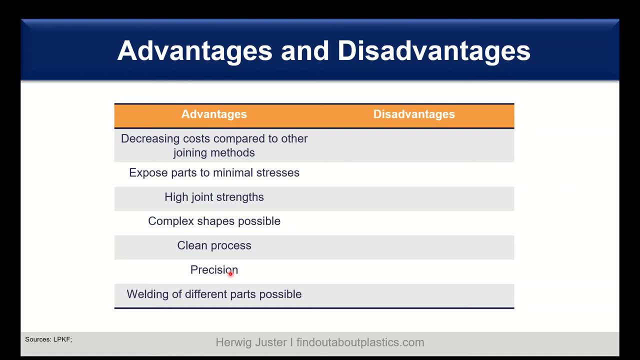 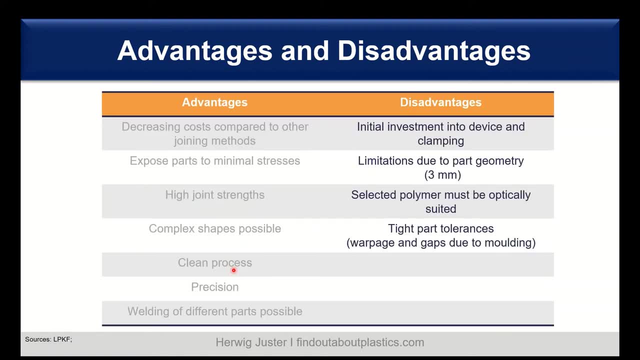 So you can have a hard to soft combination. You can have a soft to soft combination. So there are several possibilities. And what are the disadvantages? So we have, in the beginning, our first big initial investment. We need to have the laser equipment. 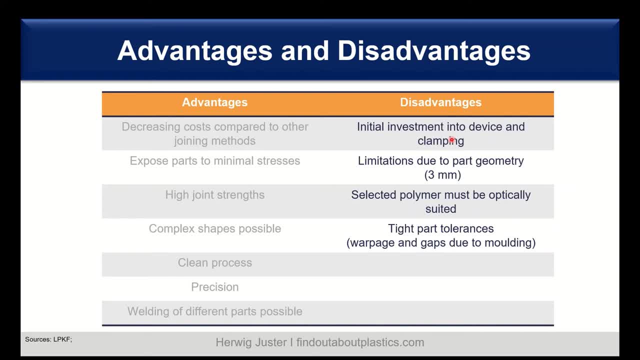 The device and also the clamping and robotics. However, then, once it is running, The costs are much lower. Then we have some limitations due to the part geometry. So when we have thick parts like 5 mm, This is already difficult for the laser to cross. 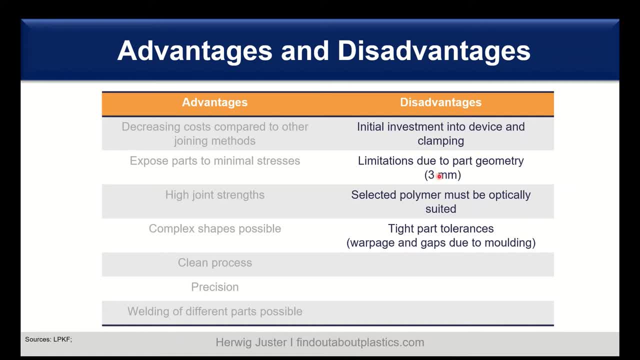 So we have here as a rule of thumb, 3 mm as a maximum thickness And, what we also already discussed, The selected polymer must be optically suited, Optical in the sense for infrared, And we also have to be careful with the The part tolerances. 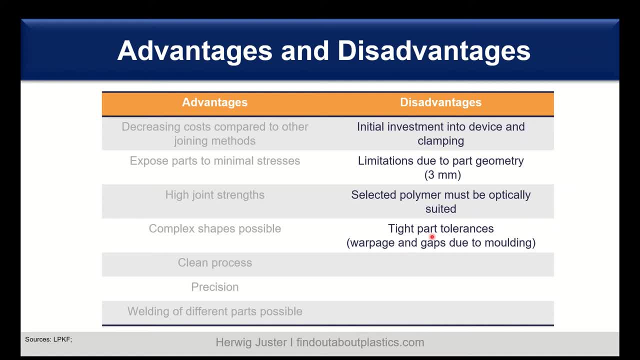 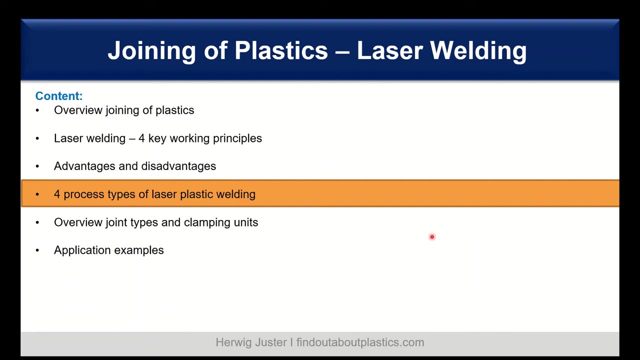 Like when we have a flat part And we have some warpage Then or gaps due to the molding. This can be a disadvantage then in the laser welding And not a conform uniform weld. Okay, Let's continue with the four process types of plastic welding. 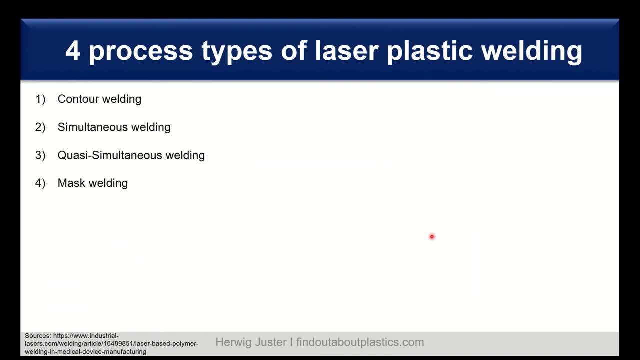 So we have the contour welding, We have the simultaneous welding, Quasi simultaneous welding, And the mask welding, So contour welding, the name already is saying it. So the laser beam is focused on a, Into a point and follows the contour of the part. 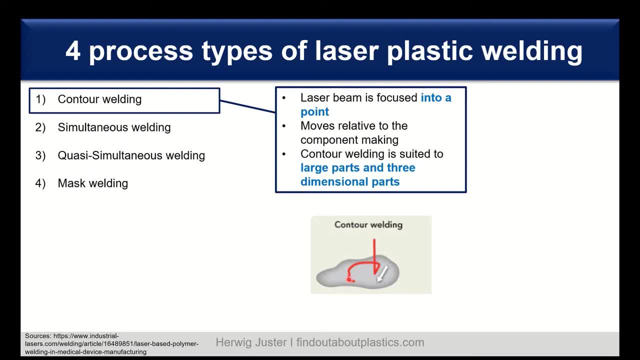 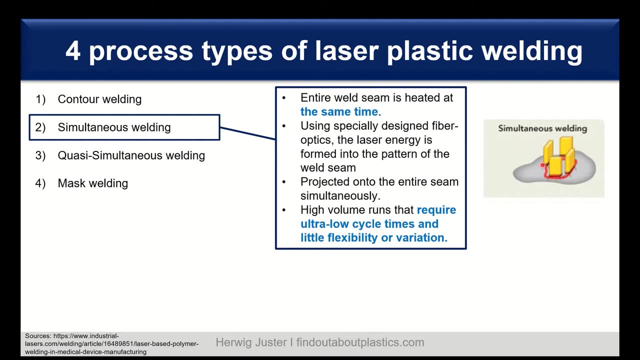 Which needs to be welded, So it moves relative to the component. So when you have the advantage, when you have large parts And also three dimensional parts, Then the simultaneous welding Here the entire weld seam is heated at the same time. So they use specially designed fiber optics. 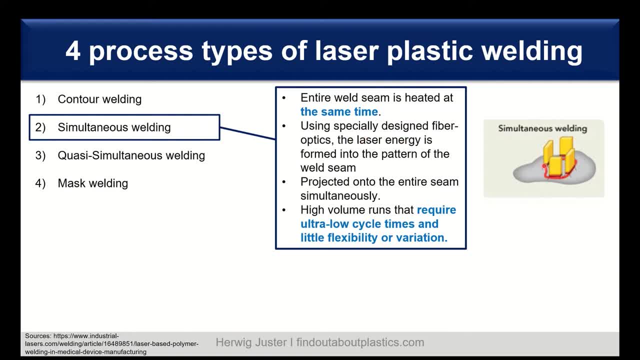 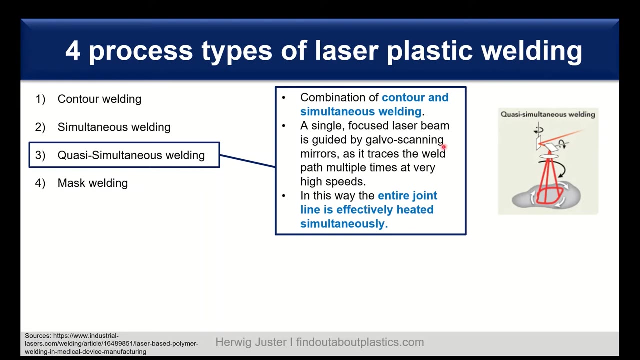 And you can transfer the laser energy Into the pattern of the weld seam. It's an advantage when you have high volume runs That require a really low cycle time And little flexibility or variation. Then we have the quasi simultaneous welding. So this is a combination of contour and simultaneous welding. 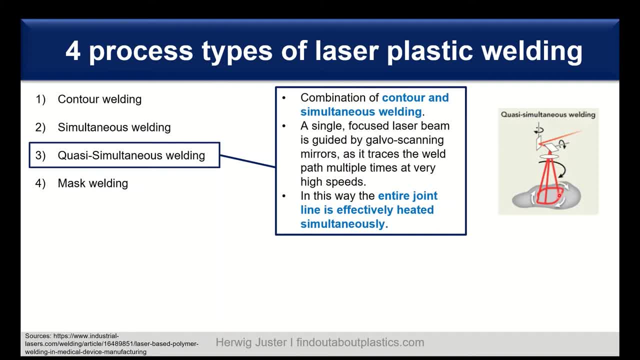 So you have again a single focused laser beam. However, this is guided by a galvo scanning mirrors, As you can see here, And it allows that the entire joint line is effectively heated Simultaneously and welded. Okay, And then we have the mask welding. 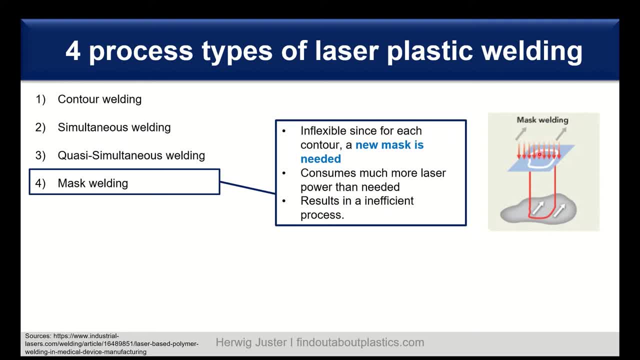 What you can see here in blue. This is a mask with the contour of the part which needs to be welded. However, the whole area is exposed to laser, And so it's not really an efficient process. You need always a new mask for a new part. 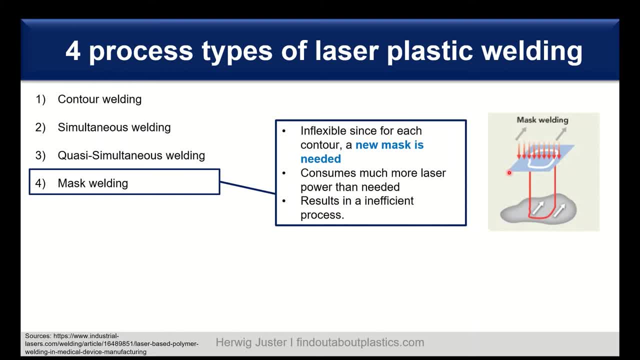 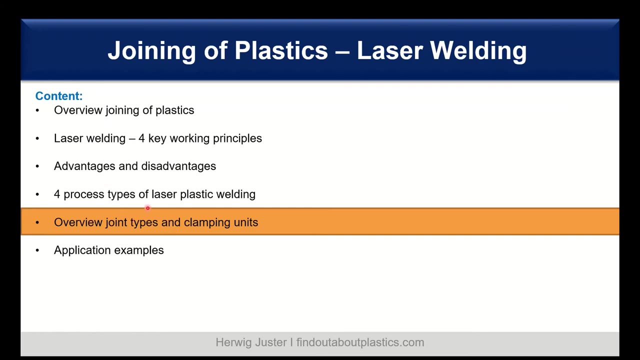 And you can imagine you need much more laser power Than actually is needed to make a simple contour. So among those four, It is more the contour, simultaneous and quasi simultaneous welding Which are nowadays in use in industry. Okay, Let's discuss the joint types and the clamping units. 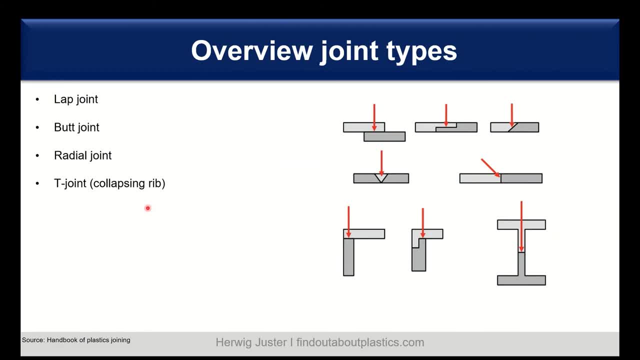 So there are again several possibilities How to joint two parts together And I have listed here the four major joints. There are several more in the literature. However, most common are lap joints. So you can see here We always have an overlap of two parts. 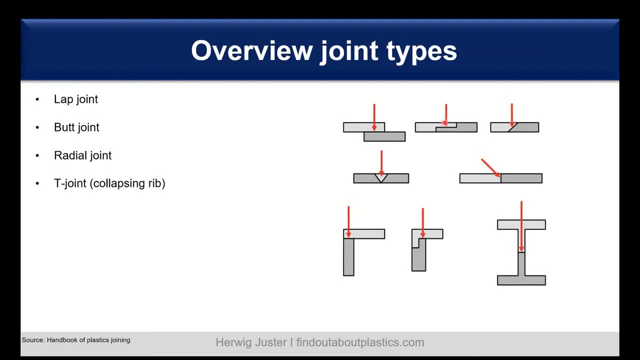 And in this overlap We focused on the laser beam And have the welding line here. We have also butt joint, For example. it is shown here. It is much more difficult, Also in terms of the clamping unit, To hold those two parts together. 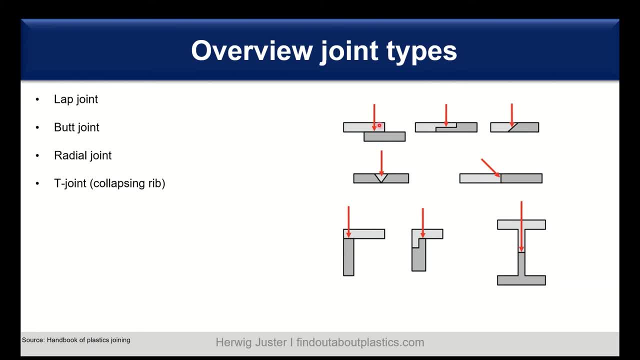 We have radial joints, Similar to the lap joint, However in a radial, When you have a curvature And like, for example, A drinking glass. And then there are also the T joints, Where the absorbing part Has a rip, And this rip is then. 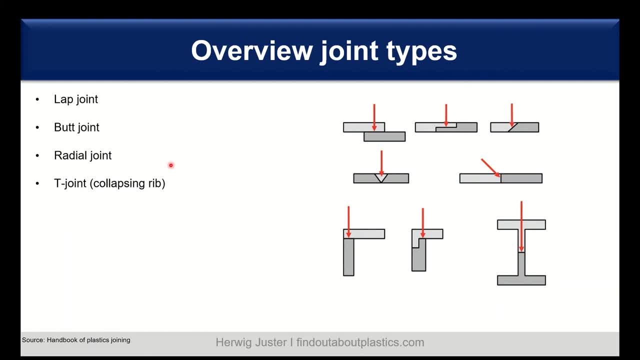 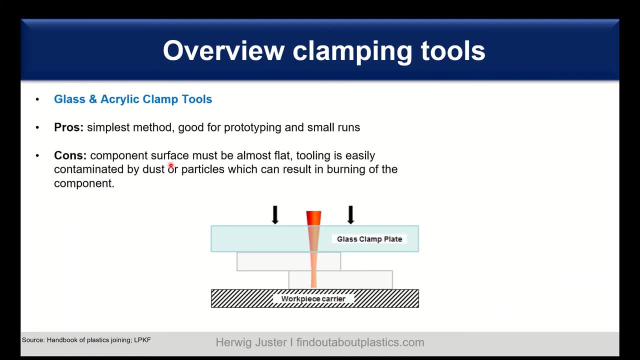 Due to the heat And the melt: Collapsing And joints, Then the outer absorbing layer, Transmissive layer, Then clamping tools. So to realize a joint, We need to clamp the two parts together first, And the most effective and simplest way. 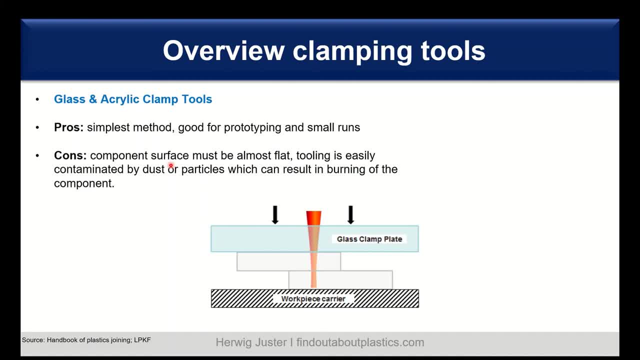 Is glass or acrylic clamping tools. It is shown here. So we have our work piece carrier, We have our absorbing layer, Our transmissive layer, And then we have the clamping layer, Which is here Made out of glass, So the infrared. 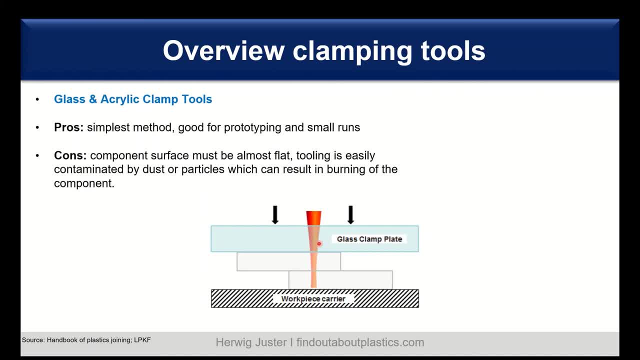 Has no problem to go through here And go through the transmissive And then to the absorber layer. Simple method, Good for prototyping and small runs. Downside is The component surface Must be almost flat And there is the risk. 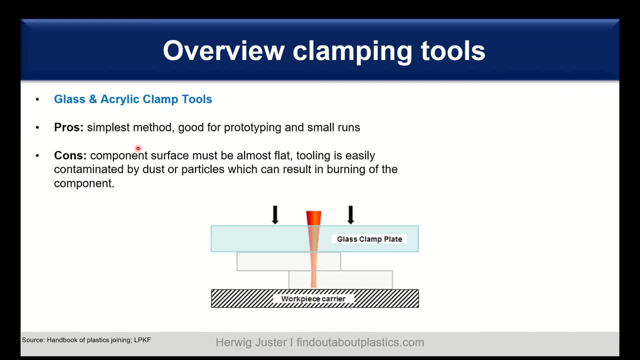 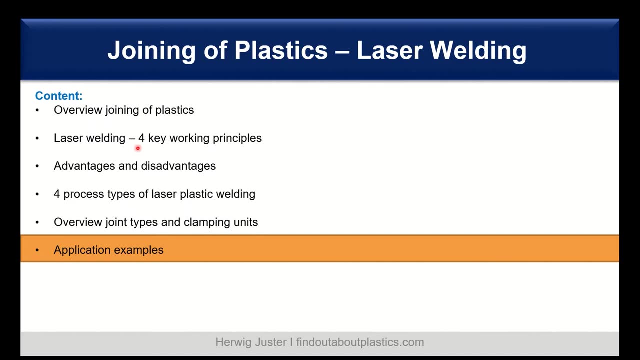 That the tooling is easily contaminated By dust or particles. This can As a result of the Burning of the component. Okay, Now We discuss some applications Of laser welding. So here You can see a camshaft sensor. 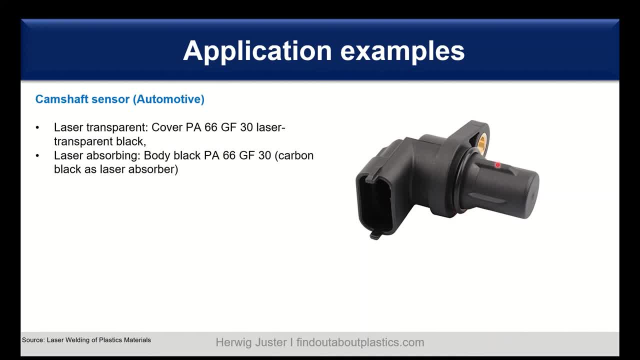 Out of automotive Market. We have here The, The cover, And this is A Laser, transparent, Black, Polyamide 66. With 30% glass fiber. And then we have the, The body, Which is our absorbing layer. 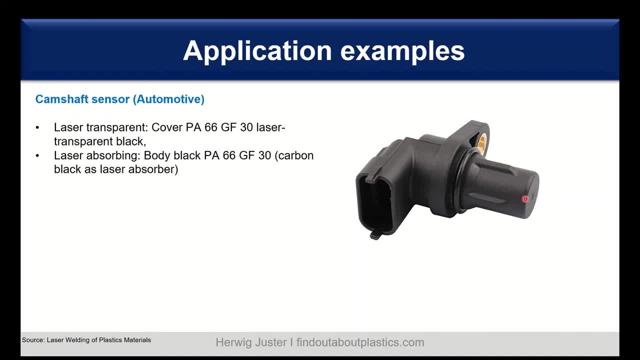 And the cover Is the Transparent layer And the body Is also A P66. Glass fiber 30% And with carbon black As a laser absorber. So We have here The The Cover.